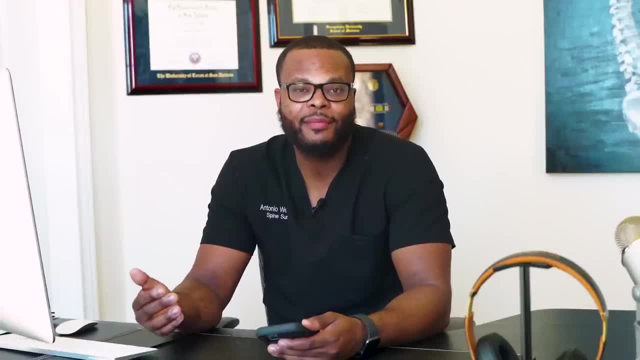 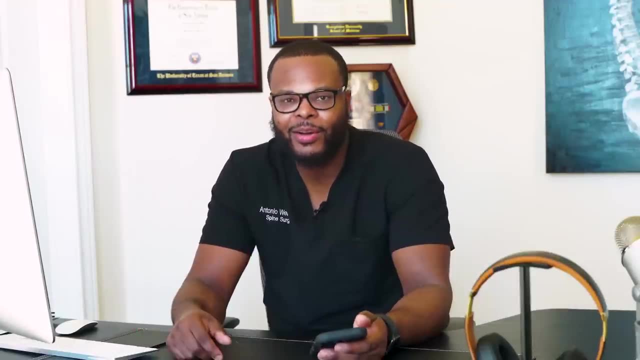 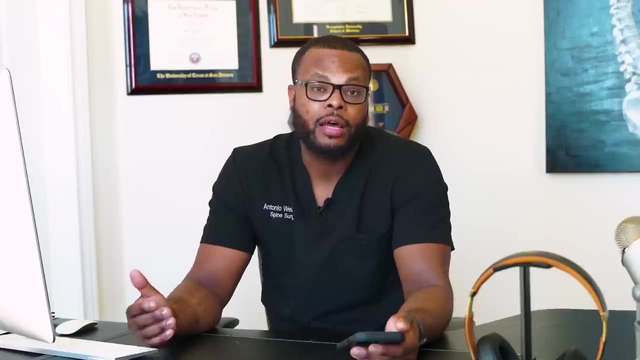 these numbers actually real, The numbers that you see out there about how much doctors make? they make all this money they have. you know, these big houses, nice cars, they do really well- Is that actually true? So, from someone who's been in private practice for one year- I just started my 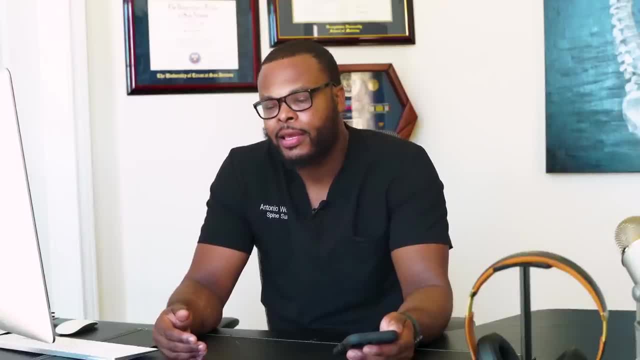 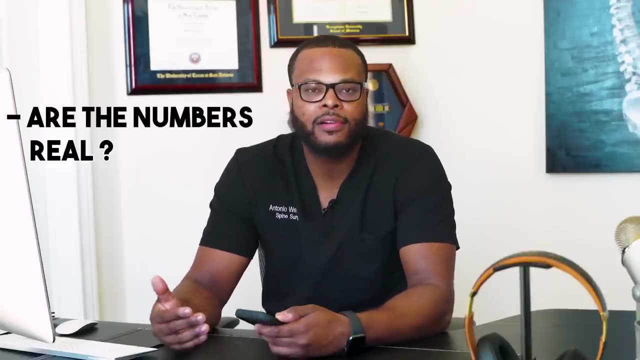 second year in private practice here in San Antonio, Texas, and I just wanted to let you guys know: are those numbers real, Is it really close, Are they really off on these estimates And what can people kind of generally expect to make Some? 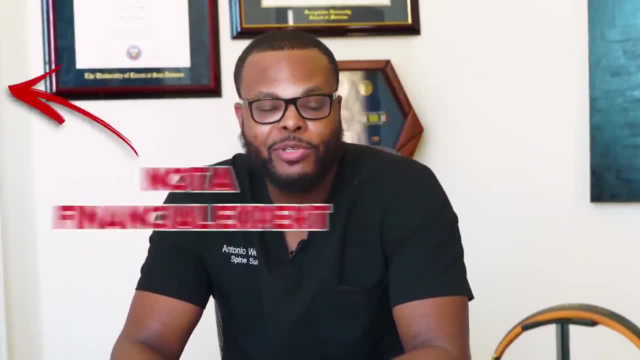 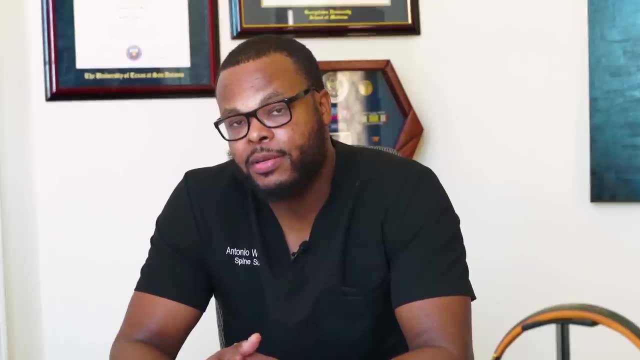 disclaimers. I'm not an expert in this. I don't claim to be an expert, You know. this is just my experience of being in medicine for the last number of years, as well as been in private practice for the last. 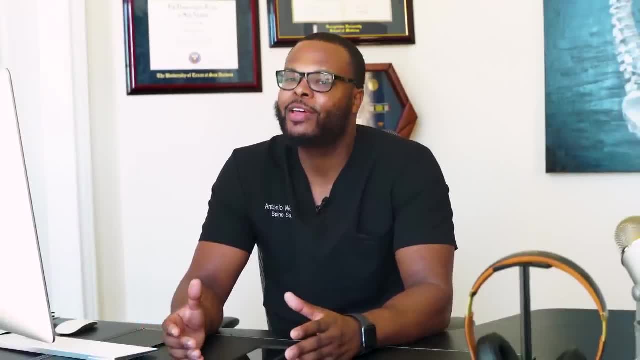 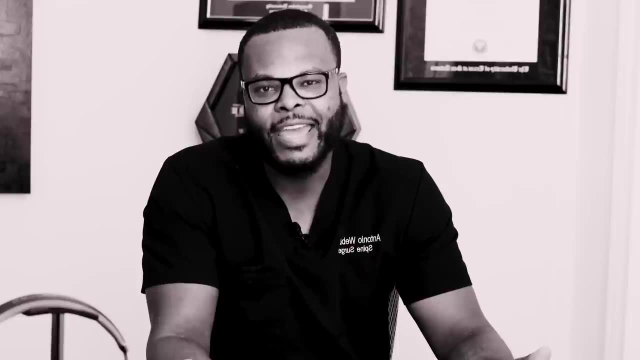 year. Also, there's gonna be people that are gonna say: oh, I know a nephrologist who makes three million dollars per year. Oh, I know a pediatrician who makes eight hundred thousand dollars per year. Totally fine, I mean everybody's salary. 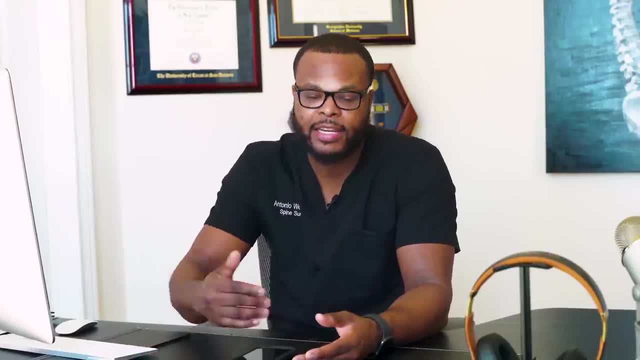 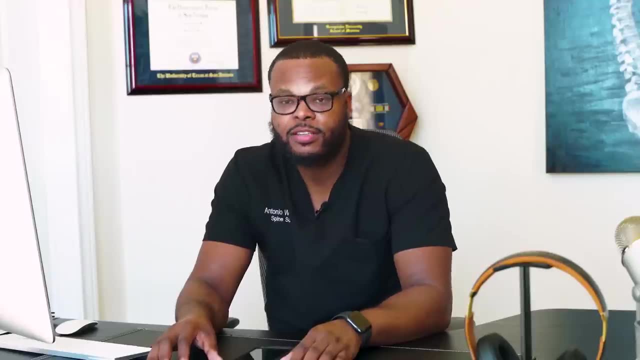 is different depending on your practice type, what part of the country that you're located. If you're in private practice, academics or an employee position. if you have ownership into your business, if you own your business, if you have other generating forms of income, it would vary. There are some pediatricians who make more than spine surgeons and there are some spine surgeons who make more than dermatologists. And there are some physicians in the same group, also within the same practice, same specialty. One makes a million dollars, other one makes two hundred and fifty thousand dollars. a. 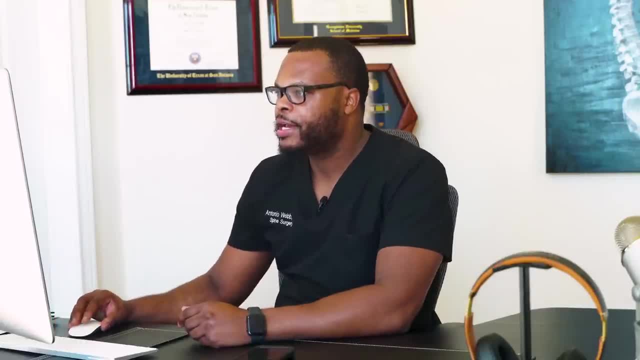 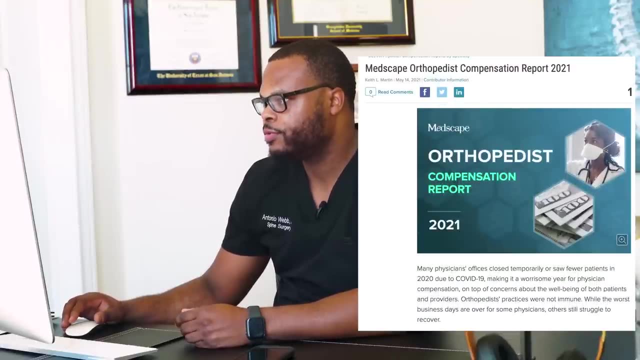 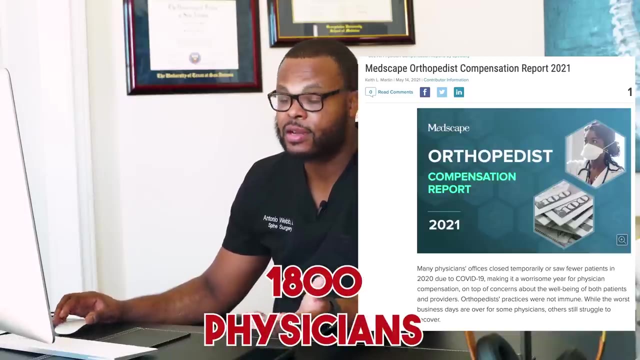 year so it varies, but there is, uh, this medscape article that always comes out every year that that usually interviews and surveys physicians. so this one is for 2021, the medscape article that came out. they asked over 18 000 physicians, so it's really widespread and over 29 specialties. about their income and, as expected, usually always at the top of the list is orthopedics. five hundred and eleven thousand dollars, so this is a kind of a median or a average income. some people made more than this. a lot of people made less than this, but 511 000 for these surveys and 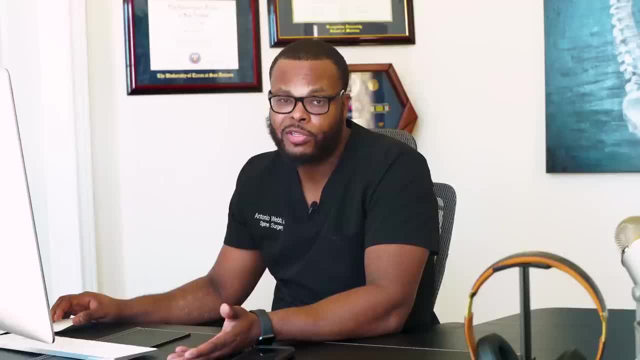 i've mentioned this in other videos. they never include spinal surgery or neurosurgery in this, just because i think they don't get enough responses when they send out these surveys. they're the neurosurgeons are probably busy, uh, operating on brains. i don't have time to respond to these. 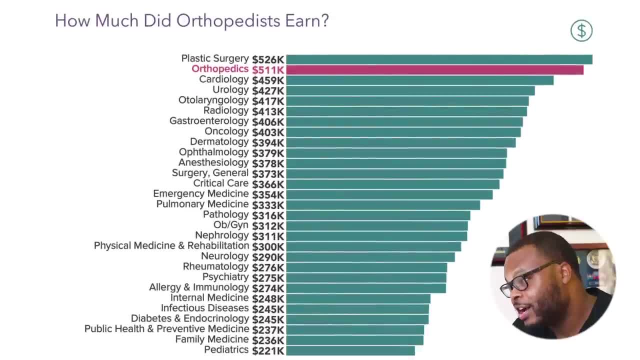 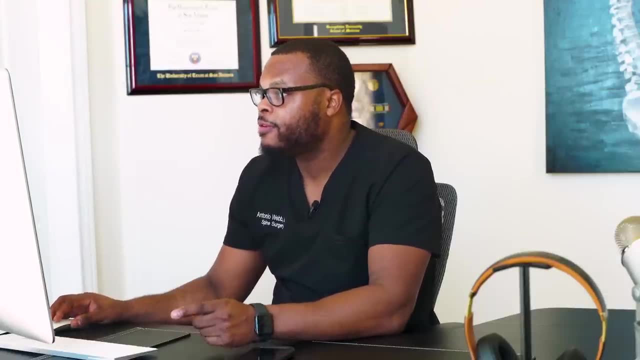 surveys. but plastic surgeries is up uh 526 000. third on the list is cardiology at 459, and then you have urology ent radiology. so is this number um really accurate? well, before i answer that, um, if you go over to salarycom- and this is not something that i would recommend, kind, of um, you know, basing your decision or trying to see how much a, you know a orthopedic surgeon makes, and they report that the median income, you know, is five hundred thousand dollars. so this is actually not far off from what medscape reports. uh, the gentleman in the, uh, the instagram message also. 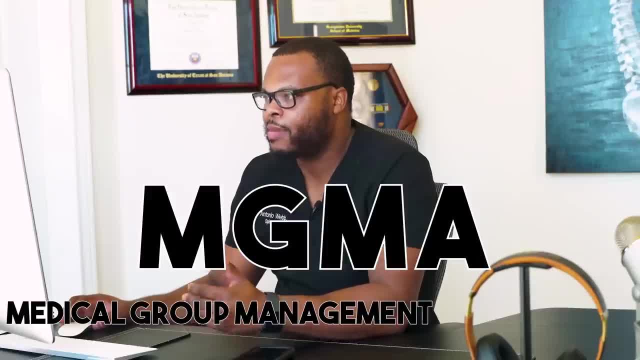 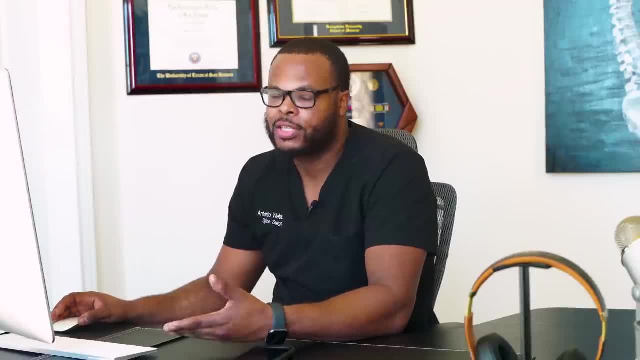 we mentioned the mgma, that's, the medical group management association. these are essentially figures kind of across the us about how much what's the average pay for a physician. so i don't have that data. just because it was kind of hard to uh yeah, and then i just wanted to kind of 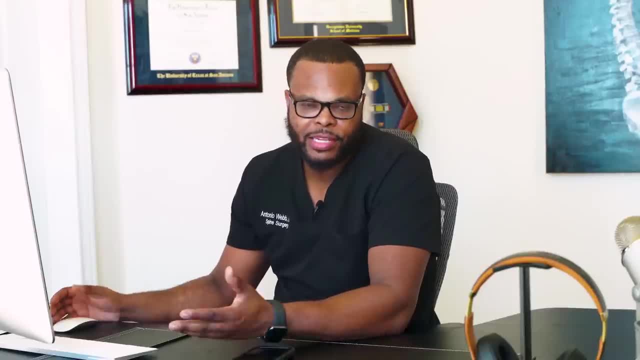 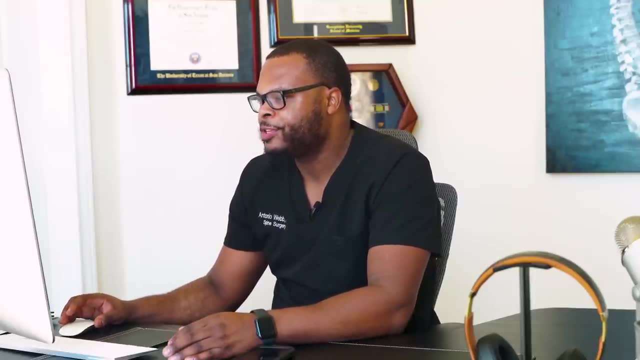 kind of get into their system. But it essentially would show around $500,000.. So the Medscape was a $511,000.. The salarycom was $500,000. And then the MGMA would depend on what part of country that. 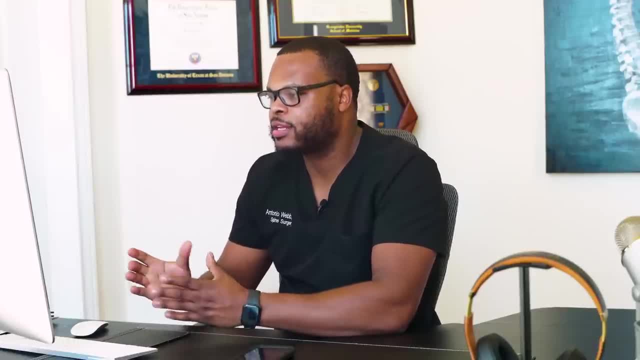 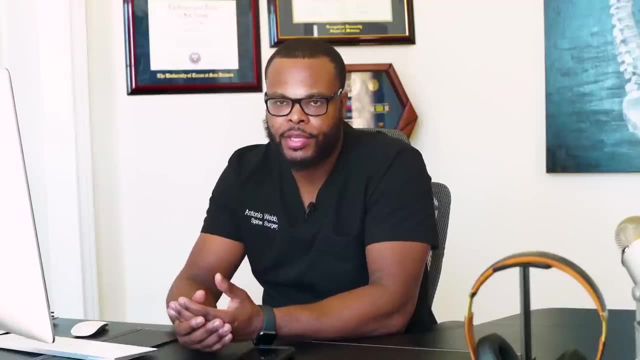 you're in what, your practice type and all those things. So there's a lot of things that come into play. So the question is: is this number accurate? And I'm not going to talk about the average for a spine surgeon. It varies. There's some figures out there. if you Google the salary of a spine. 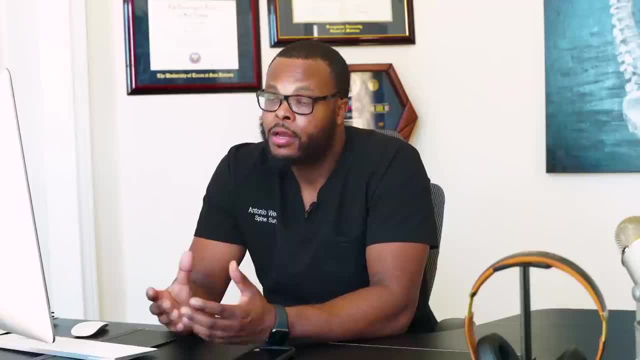 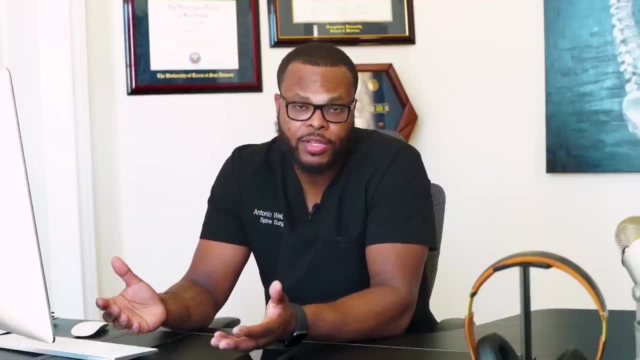 surgeon. But I think orthopedic surgeon is kind of more something more easily to talk about in terms of salary And just because I have a large percentage of my practice that is orthopedics, I do take general orthopedic trauma call, So I do see patients with general 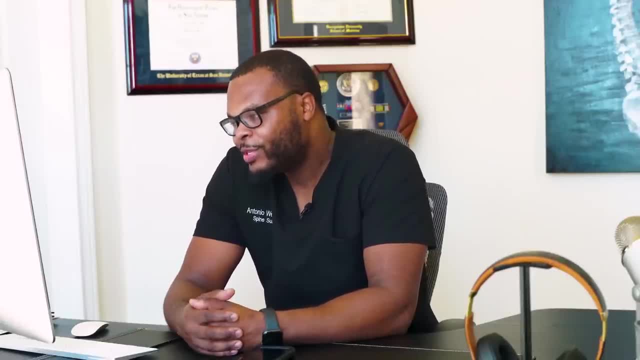 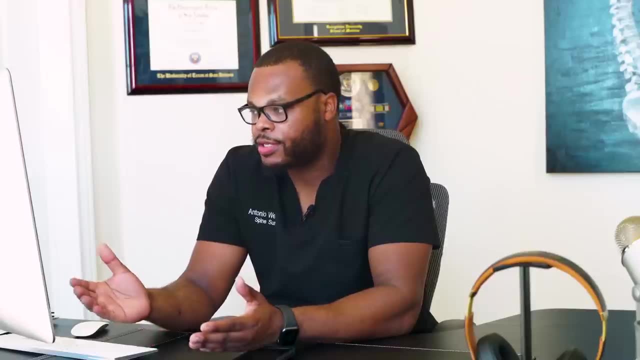 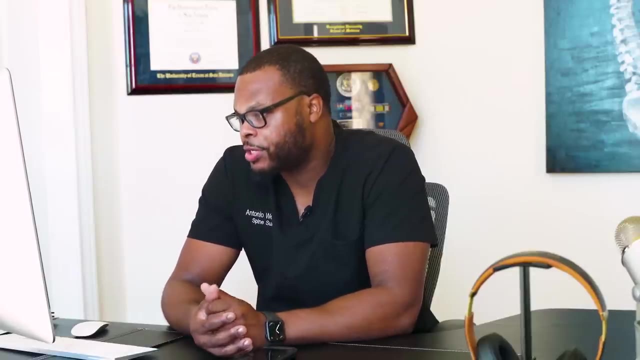 orthopedic complaints as well. Is this number accurate? I would say this number yes And no, So $500,000.. This is a 50% medium on salarycom. Is this number pretty accurate after being out in practice for the last year? One caveat is that COVID COVID has definitely 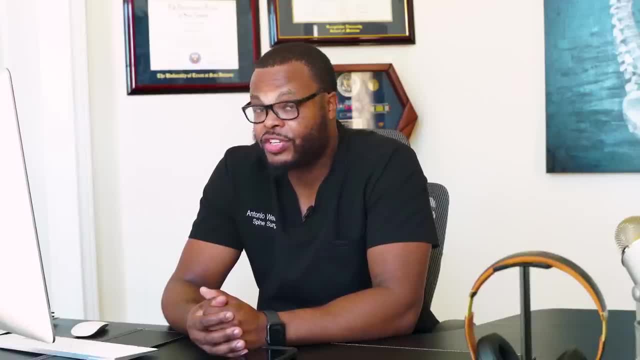 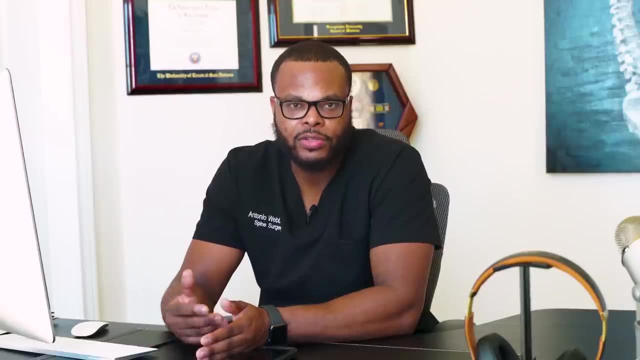 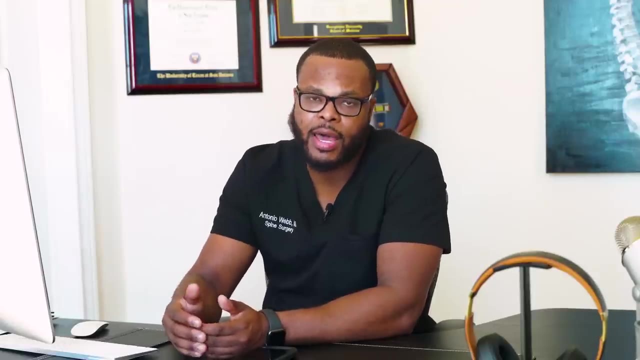 impacted the salary and compensation of physicians across the board. The numbers that are reported now may not represent what they were pre-COVID, So 2019, 2018, 2017.. So the most physicians have seen a decline in their salary, Although there are some physicians that have seen an. 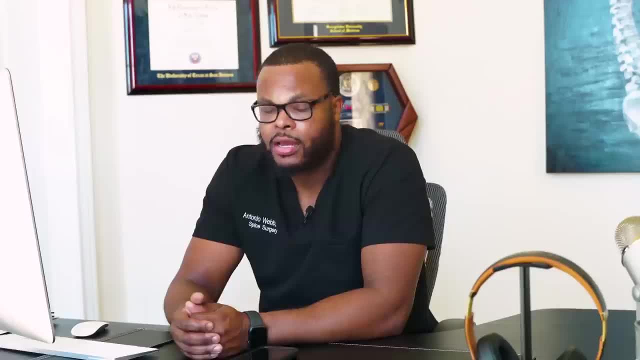 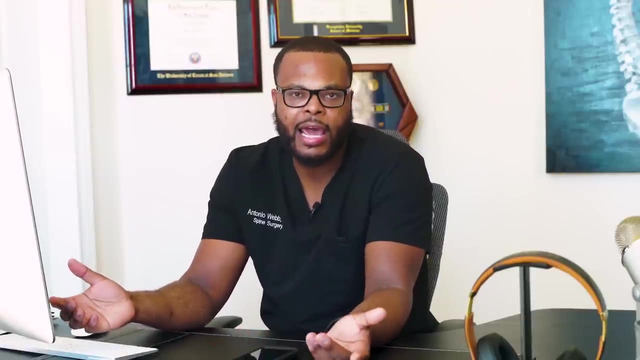 increase. So across the board, most physicians have seen a decrease in their salary. Before I answer the, is this number pretty accurate? There are a couple of different ways of practice models that physicians can join once they leave your training, And I've made other videos about. 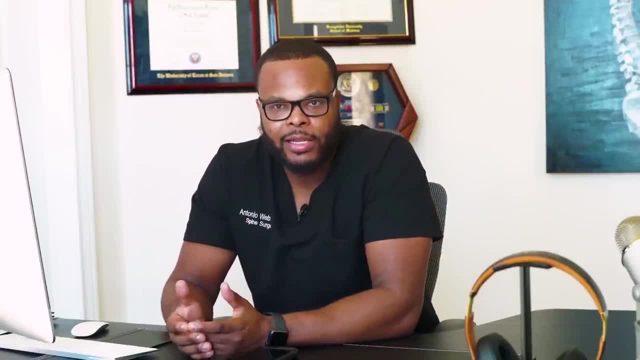 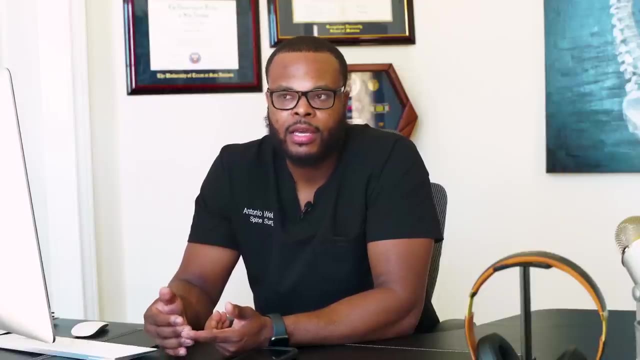 this. I'll put that right up here, But real quickly, a physician can join a practice model where you can go into an employed position, which means you work for a hospital, essentially, and the hospital pays you a salary, or they can pay you based off of what's called productivity. 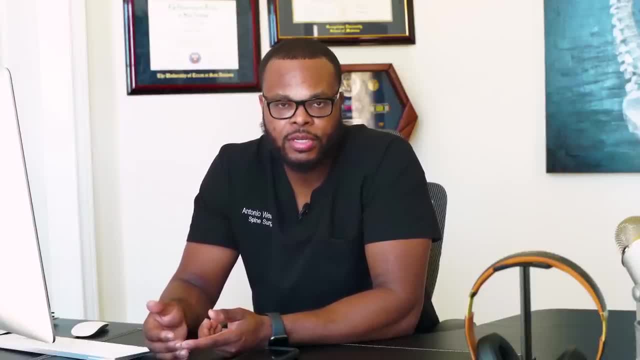 The more work that you do, the more patients that you see, the more surgeries or procedures that you perform, the more your salary will be. But most of the employed positions- if you think about being an employee at a hospital, this is usually a salaried position And then 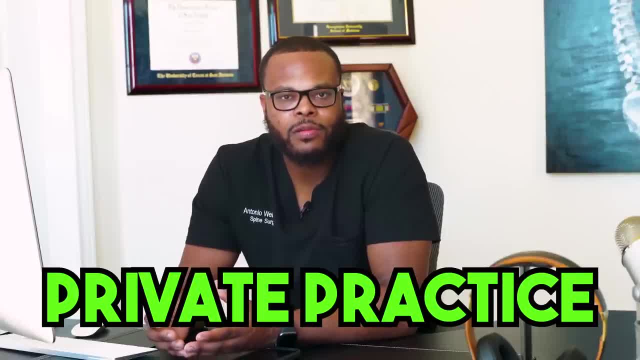 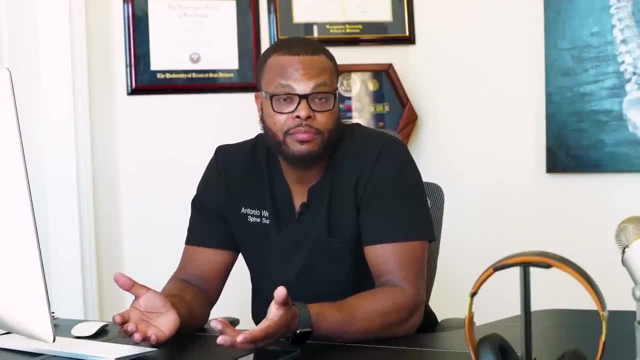 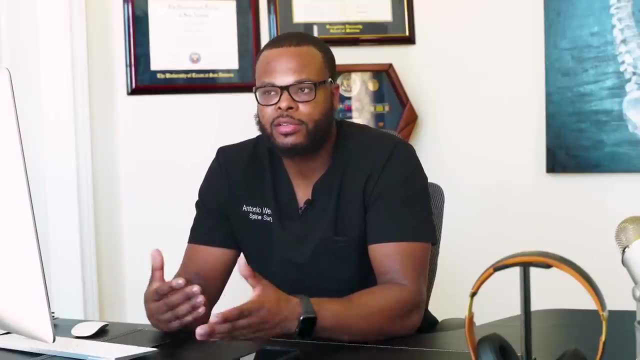 there's private practice. Private practice: either you join a group of other physicians who had their own business or you start your own business and essentially in medicine- And it's for most- people are kind of what's eat what you kill. This is essentially the more surgeries, the more patients, the more. 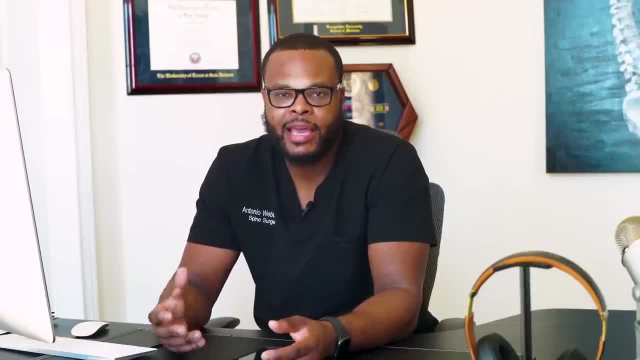 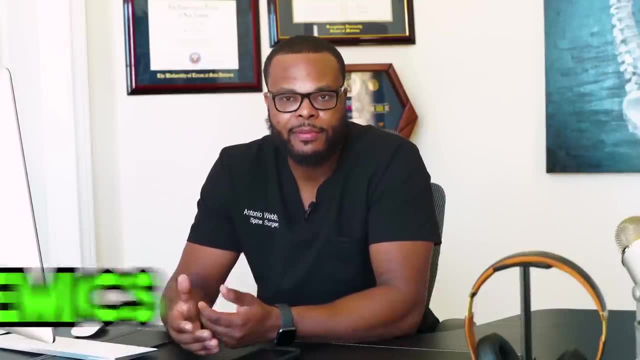 procedures that you do- the more diagnostic tests, those things- the more you will get paid. And then there is academics, which means you work at a university or some type of setting where you're teaching medical students. And then there's the private practice, which means you work at a 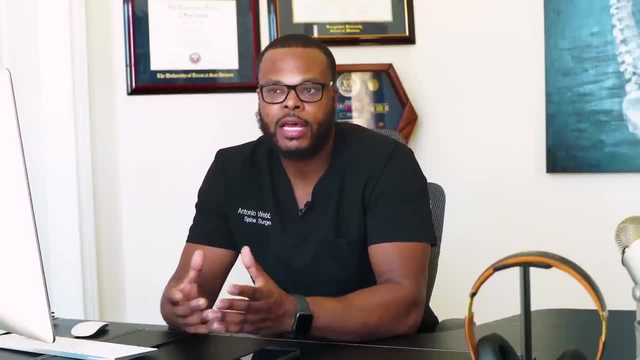 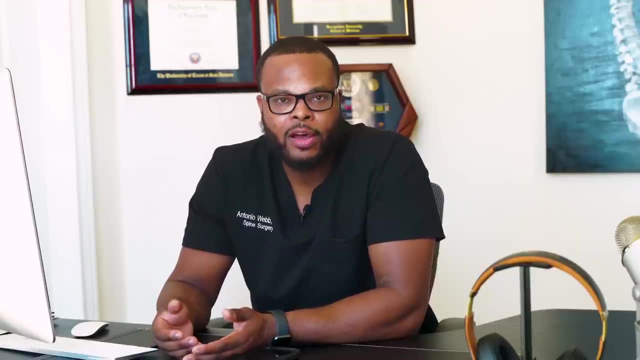 student's residence. you get this appointment ship, which like clinical professorship, and that's usually salaried as well. But there are some productivity incentives to work at an academic center. So the salary will depend on your practice type, what part of country. that you're in and also your specialty. So this number- $500,000, I do believe this number is pretty accurate. It's for the first year. You know, most orthopedic surgeons, depending on what part of country that they're in, are around that kind of range. But if you're fresh out of practice, especially in private practice. you have to build your practice. That takes time, Just like if you started a business. it's going to take time to generate your practice, your clientele, your patients, and to generate this much money. It may take two to three years. many times, sometimes Four years. There are some surgeons that go out and practice and they get busy really quickly and they can make $500,000, $600,000, $700,000, $800,000 per year. There are some other surgeons-